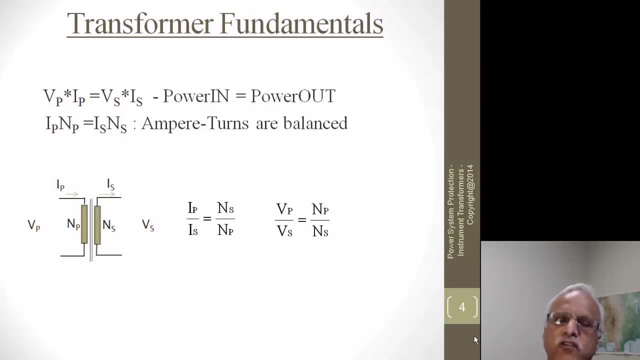 Before we get into the current transformers, we look at the transformer fundamentals. whether it is a voltage or a current transformer, The power into the primary winding will be equal to power out. So VP times IP must be equal to VS times IS where P is the primary winding. 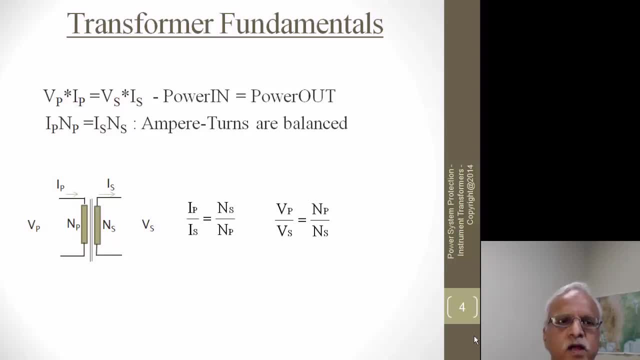 The Wilder's is the secondary winding And then the Ampere turns must be balanced, That is, IP times NP must be equal to IS times NS. So if you take a look at that, then the voltage ratio from primary to secondary will be the same as the turns ratio of the transformer: NP to NS. 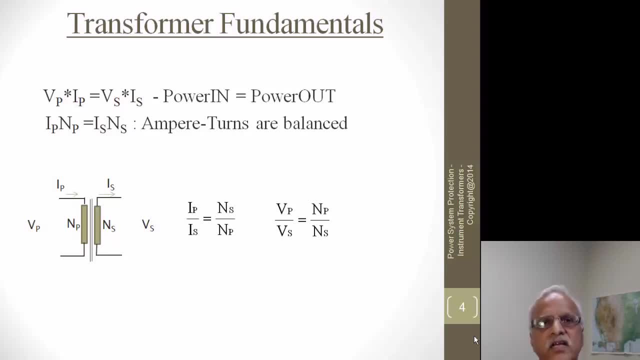 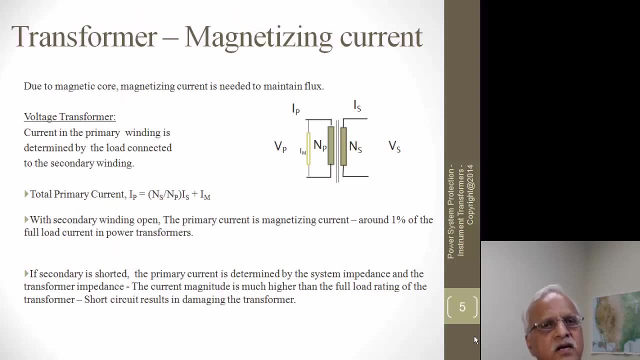 And then, whereas the current is equal to inverse of the ratio of the transformer, So IP by IS equal to NS in p. and then, because you have a magnetic cup core which is linking the two magnet, two windings, you need some energy and the current in maintaining the flux linkage. and then this: 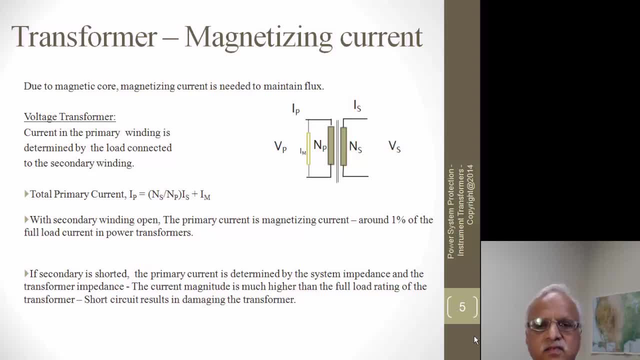 is called the magnetizing current and then, as we mentioned it here, it is only one percent of the rated current of the transformer. and then you know if you find a relationship. in a voltage transformer, the secondary current is just voltage on the secondary side divided by the amount of ohmic. 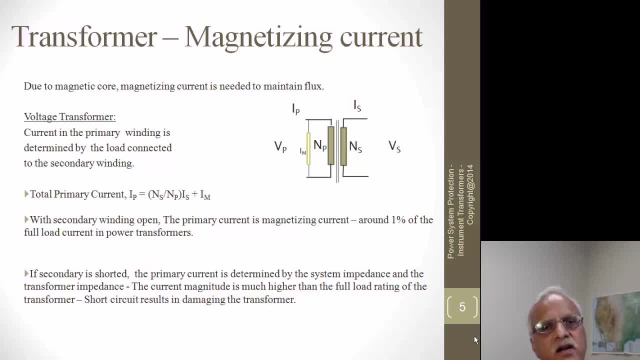 burden. that is connected ohmic load burden and load. i will be interchanging it very often. it is just the load connected on the secondary side is we call this burden in trans instrument transformer vocabulary. so the current is just a voltage on the vs divided by the load and that is is and that is. 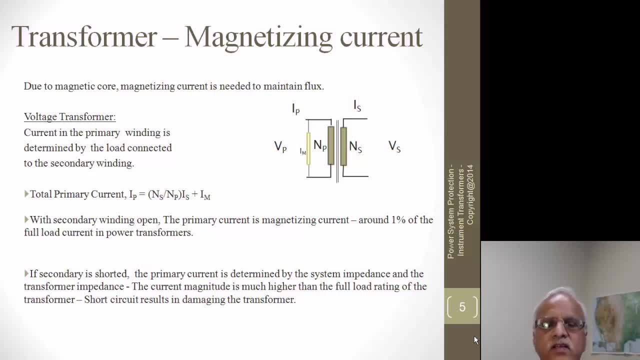 reflected on the secondary side of the transformer. so that is the voltage on the secondary side of the transformer. so that is the load connected on the secondary side of the transformer. so that is the load connected on to the primary side. and then we use some current to magnetize the core, so the 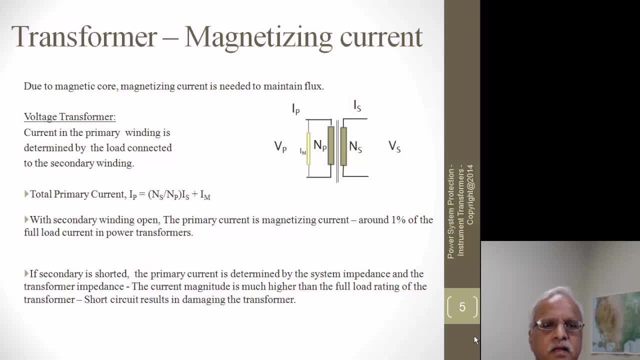 primary current is nothing but the is multiplied by, divided by the end, or you know, is multiplied by the turns ratio on the secondary side. I tie is times ns, it is ampere turns and then plus the magnetizing current, which I said is only one percent. back to this. if we keep the secondary side open on a voltage transformer, then 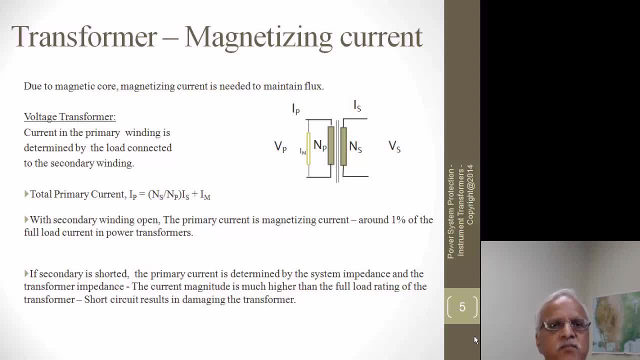 what happens here is, you will just see, a magnetizing current is flowing on the primary side, which is, as I mentioned, it's- only 1%, whereas if you short it, the short circuit current could be 10 times to 20 times the rating, normal rating of. 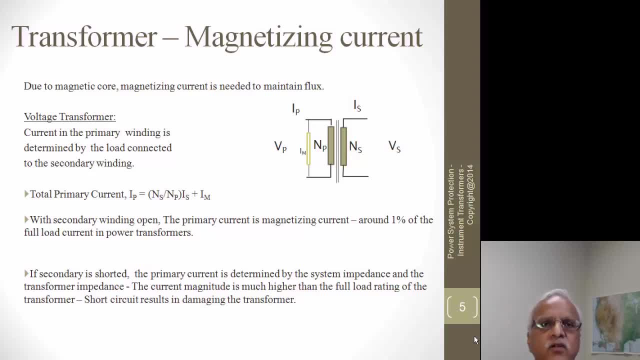 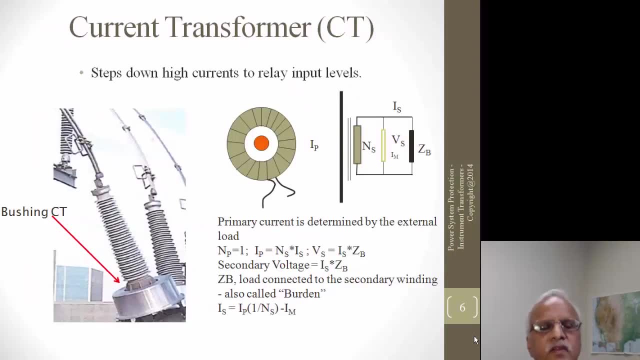 the transformer and you might damage this. the current is only limited by the impedance of the transformer between and also the source. let's look at the current transformers. in the case of voltage transformer, primary current was determined by the amount of current which is load connected on the secondary. 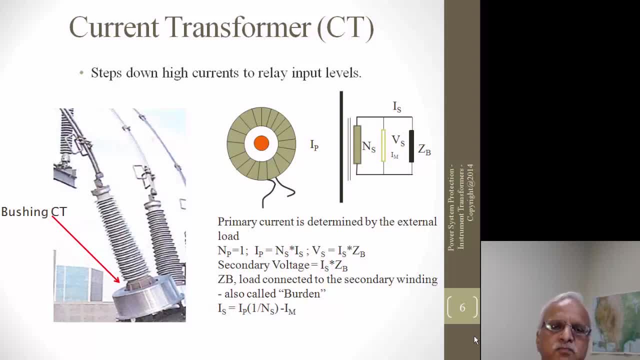 side, whereas in the case of a current transformer it is monitoring the current going on a transmission line or in it through it, or current through an equipment, so it has no control on the amount of current flowing through that. so that is you only by the external load, so you have the current flowing through that on the 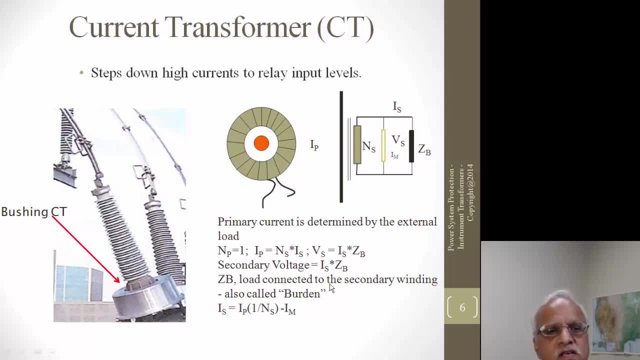 primary and normally it is only one turn, as we see here in this example, this is just the lead which is going into the breaker, which is only one turn, and you have a transformer core second out, current transformer sitting here which is mounted outside on. this is for a breaker, which is how it it is mounted. 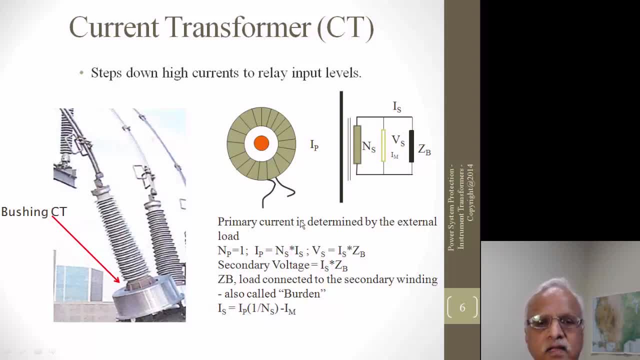 now, if you look at that, then the secondary current will be the, just the primary current divided by this and that is produced because of the ampere turns that tries to push the current through whatever burden that is connected. so if it is, if the burden is nothing but the load connected on the secondary side, 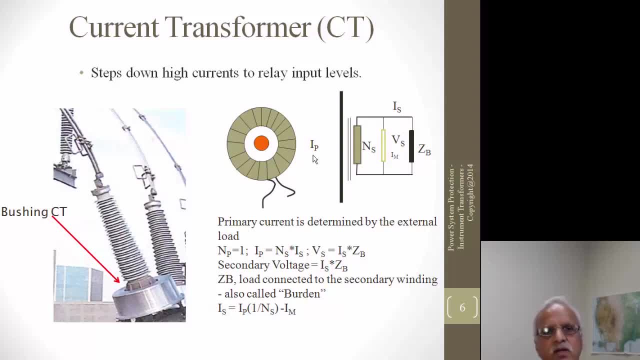 which could be a relay or a meter. so the voltage that is developed across the secondary side is is determined by you: the ohmic value of the burden multiplied by the secondary current, which is nothing but the primary current, divided by the number of turns on the secondary side. so if you short it here, what happens? it just balances the ampere. 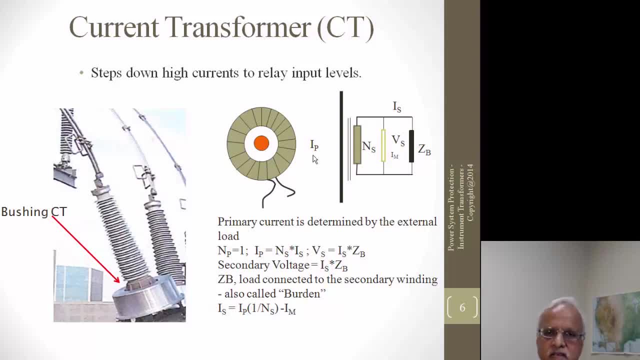 turns and there is no voltage that is developed across the secondary side. so it provides a path for the secondary current to flow, whereas if you open circuit this, the primary current is continuously going and then the secondary side. it tries to push current through an open circuit. so you get very high voltages on the secondary side and 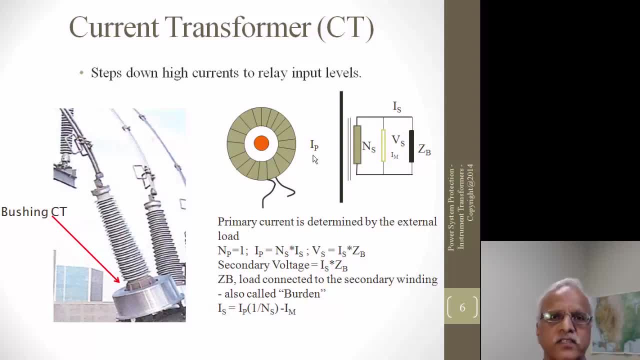 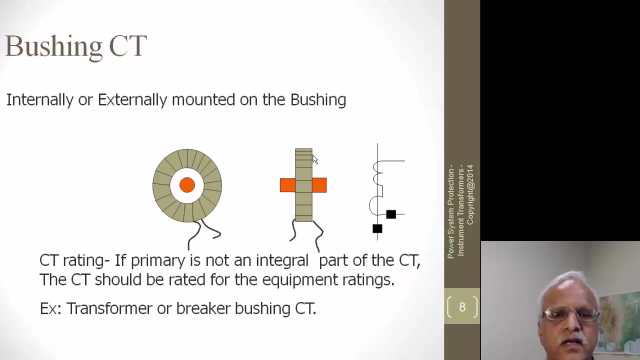 even though it cannot push a current, you get very high voltages and then the CT saturates and it gets damaged also. so in the case of a voltage transformer, you cannot short the secondary side and the case of a current transformer, you cannot keep it open. this is just a picture of that, and also the primary current is not. 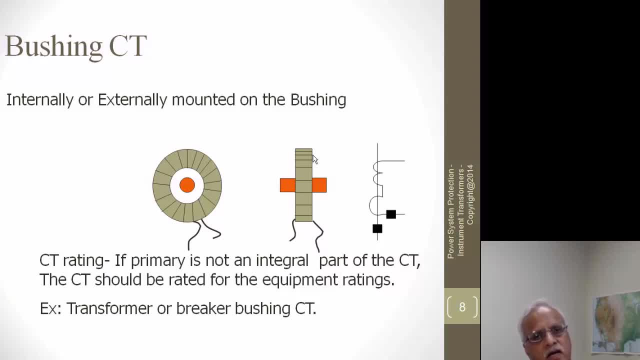 the primary rating of that is not determined by by the CT itself. you know if you are using it on a transformer, you have an ability to overload the transformer to much higher than its nominal rating, say for example 150 or 160 percent, for a short amount of time. so the CT also must be able to take care. 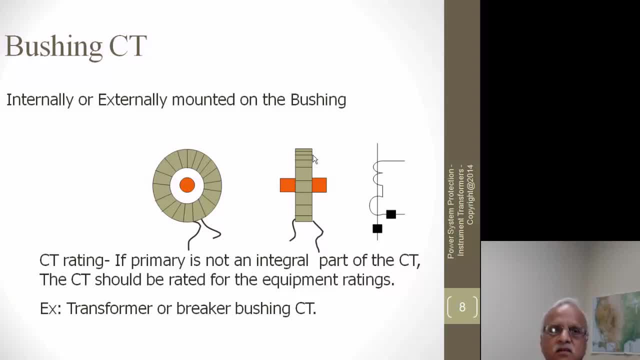 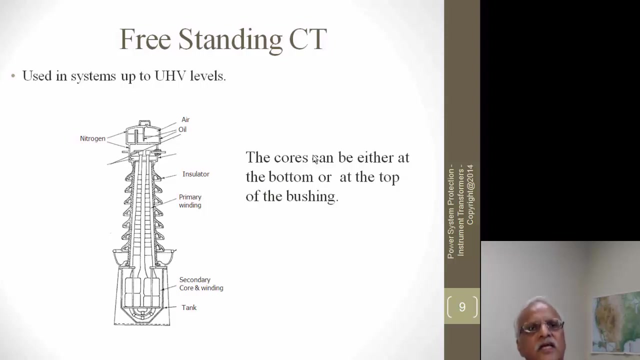 you know, must be able to carry that overload for the same amount of time. so if, because it is not an integral part of that particular, it is an integral part of that particular breaker or a transformer, these CTs also must be rated as their equipment on which these are mounted. the next one is freestanding. 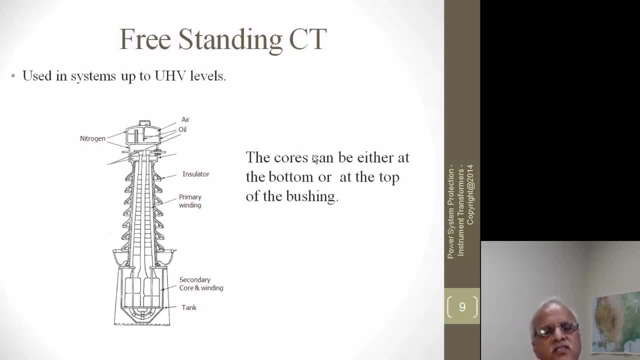 CTs. these are used on lifetime breakers where you don't have bushings. the interrupter is insulated and then it is standing by itself and there is not enough space to put the course on. there is no place for that. so you have a separate, freestanding CT on its own insulator here, if you look at it. 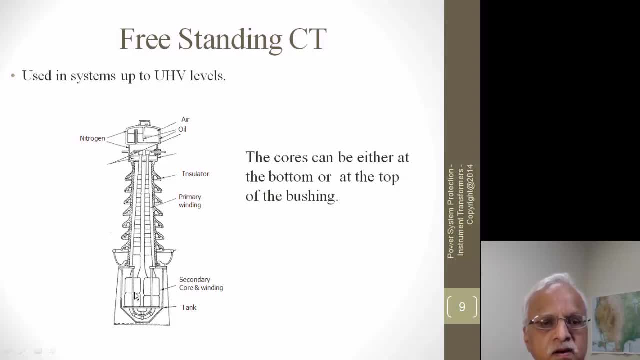 these are the primary windings. it comes down here and then goes through four cores and then it goes back. there are four cores here and the secondary windings are coming out of this. this could be either at the bottom of the tank or at the top of the tank. it depends on the manufacturer. 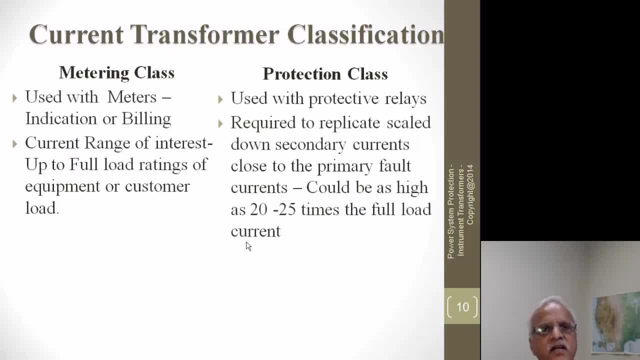 now, as far as the classifications are concerned, we have to see what is the purpose of this current transformer, whether it is used for metering or for relaying. if it is used for winter metering, that means we want to continuously monitor the load and then you know if it is billing, then you have. 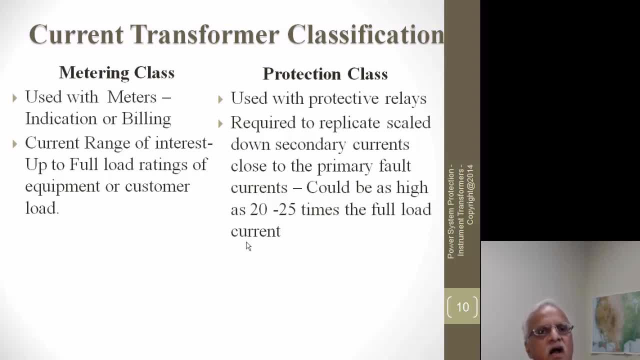 to charge them accordingly, depending on the current. so our our region of interest is from no load to full load, up to the rated current of the current transformer of the equipment on which these are mounted, whereas in the case of protection class, these are used for determining the abnormal conditions that 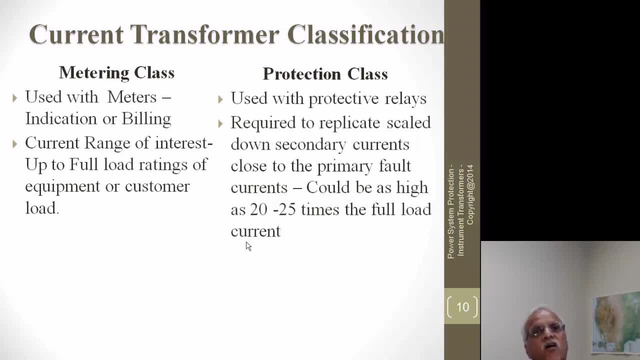 is, you know, when the fault occurs. so the fault currents could be as high as 10, 20 to 25 times the full load current. so our region of interest is not the normal operating range but the fault range where, how well, this CT can reproduce this waveform of the current transformer. so this is a very important 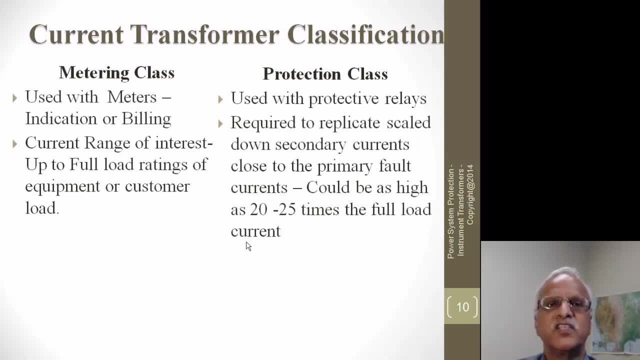 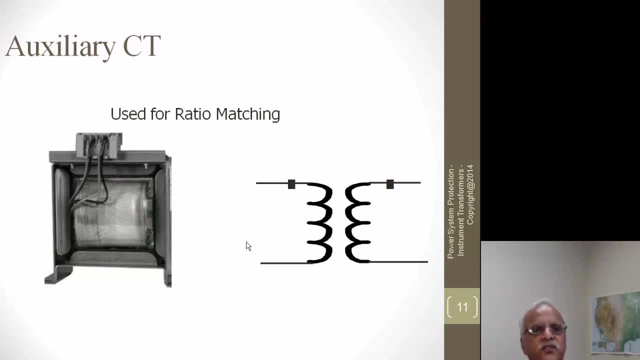 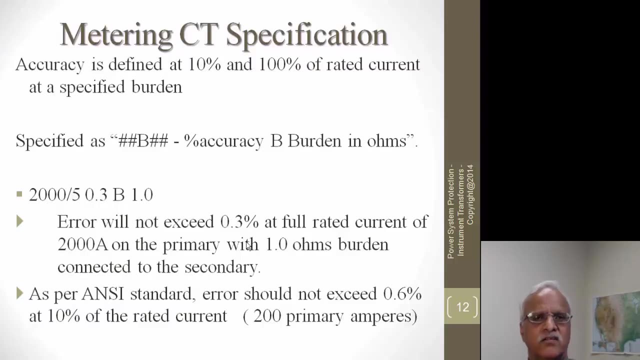 factor we need to think about. we have self-referenced a viewing Rickey photography to check that the extent to which the number of recruiters- good لهir, no, was the number i would say that we are- that the number of cut Marshall, sergey bluecher develop this relationship. we do not see any. 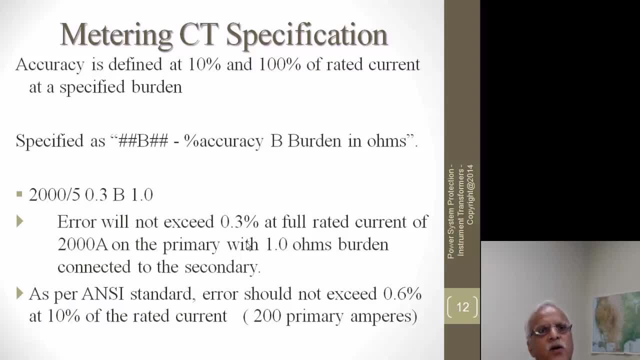 challenges down to none with that be 1.0.. 0.3 specifies the error when the current through that is about 2000 amps. This is an example for 2005.. When the current through the safety primary current is 2000 amperes. 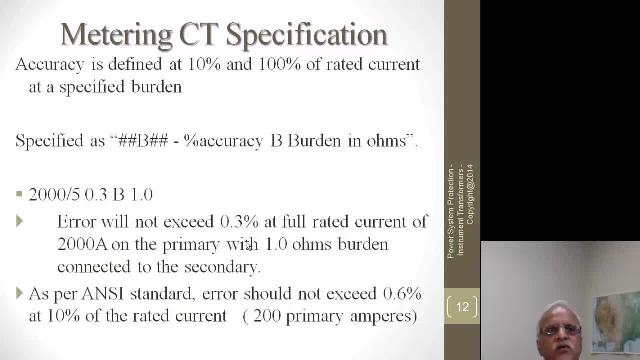 the secondary side, if it has got an unknown load or the burden connected to that, the accuracy error cannot exceed 0.3%. And then American National Standard also specifies that this error cannot be twice the specified value when the current is only 10% through. 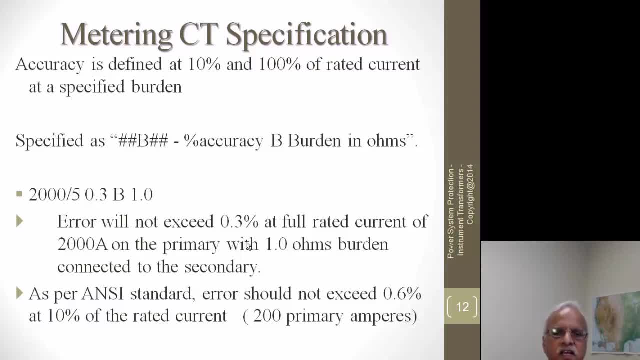 the current transformer. So at 200 amps it cannot exceed 0.6% and at 2000 amps it cannot exceed 0.3.. But this is with a burden of 1 ohm connected And also we not only worry. 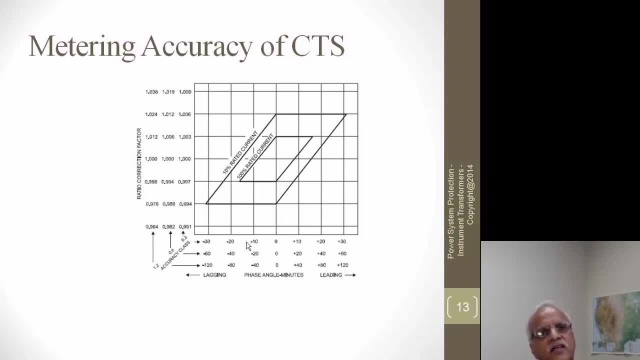 about the ratio error and we also look at the phase angle error. Suppose you are looking at the vortices- It is watts consumed by a customer, kilowatts consumed by the customer. Then you have to make sure that the current produced on the secondary reproduced on the secondary side. 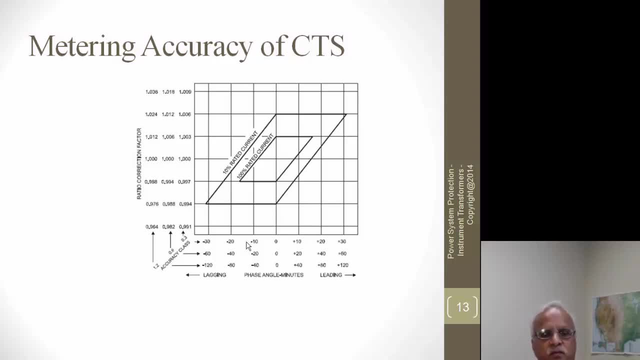 by the CT has is in phase with the primary side, So, but there are some inaccuracies, just like the ratio. You have a ratio error here and you have the phase angle error, which is the given here. This is given in minutes, So this is called a parallelogram and it is. 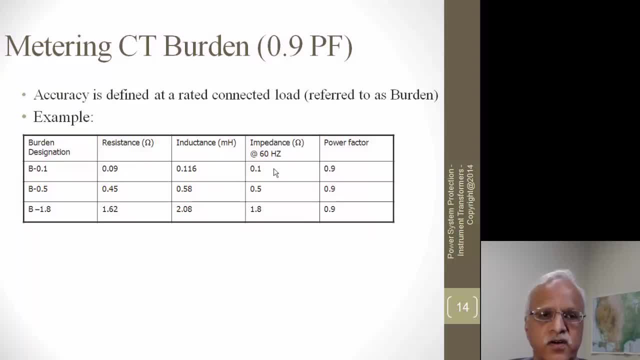 specified. it is supplied by the manufacturer. As far as the burden is concerned, a metering burden is mostly resistive. What it means is it is a little bit inductive but mostly resistive. So if it is connected across the secondary of the CT, the current, through that 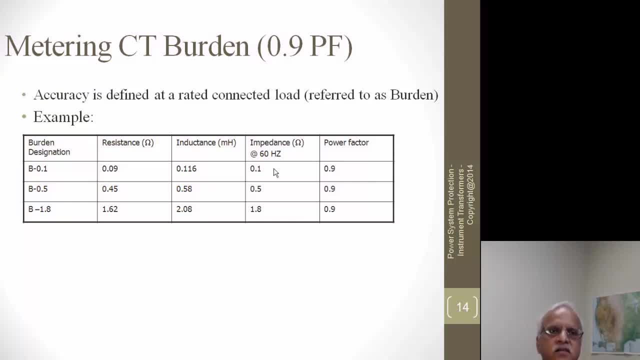 produces a voltage which is leading the current, because it is an inductive circuit and it is an RL circuit, So the current leads and relaxes the voltage by a certain angle and cosine of that angle is 0.0, 0.9.. So they have specified actual inductance and resistance. 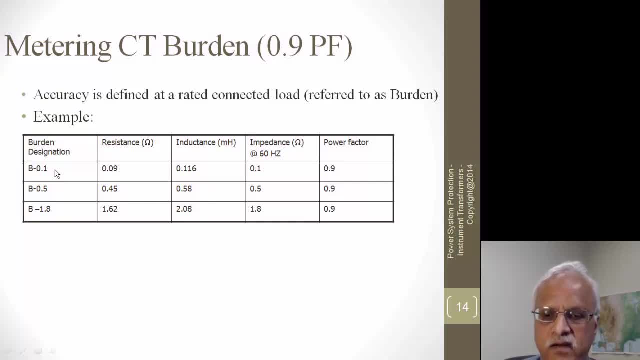 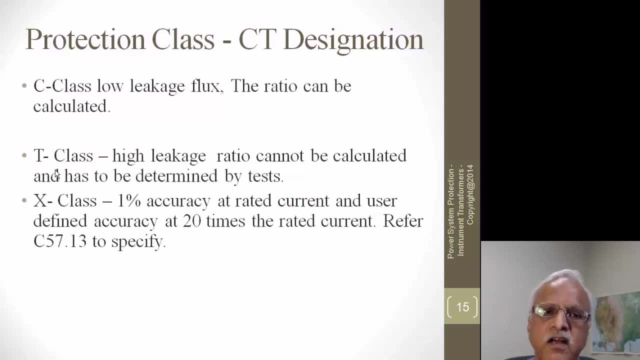 values for these standard burdens for which the CT is rated and then specified. But, as in the case of a protection class, there are three levels. One is called the C class, the other one is T class and the other one is X class. C is has got a low leakage. 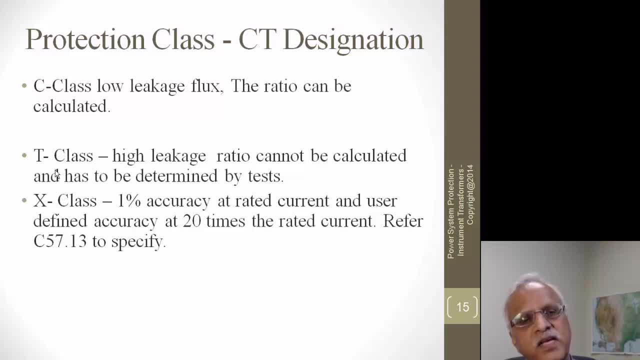 between the primary and the secondary side. So the C class has a low leakage between the primary and secondary and then the ratio can be calculated, Whereas in the T class there is so much of leakage reactance between high leakage between the primary and secondary. 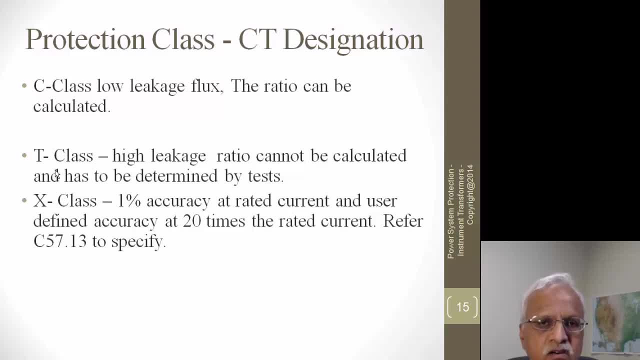 So you connect a specified relay or whatever burden you are connecting, and then you pass the current, a specified current, on the primary and calculate the accuracy through tests. And it has to be determined only through tests Most of the times protection class we use. 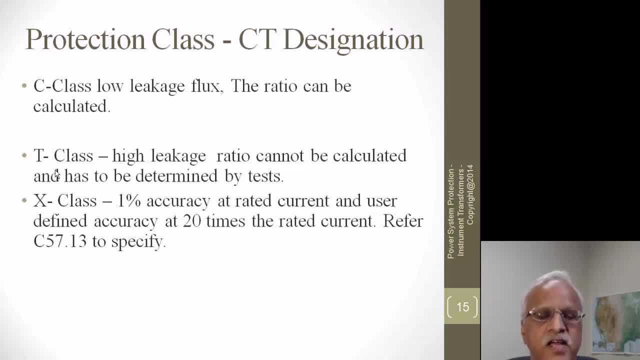 the C class In in all our applications. this is generally true, And the X class is used for 1% accuracy at rated current and then the user-specified accuracy at 20 times the rated current. This is specified in ANSI standard C57.13, IEEE standard also. It is. it is also an IEEE standard. 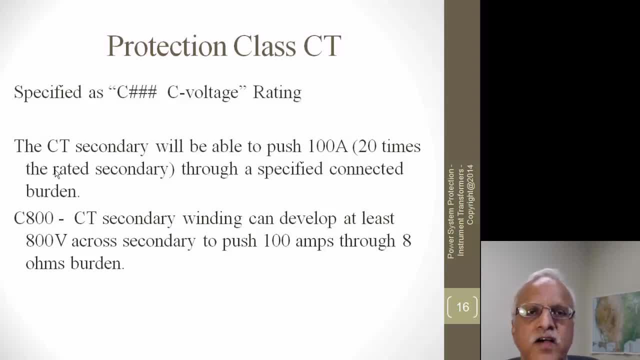 Specifying. in the case of this, it is specified as a C class and then you say it is voltage rating. It is given as the next number on that. An example here is C800.. What it means is the CT when can produce 800 volts on the terminals of the secondary when 8 ohms is? 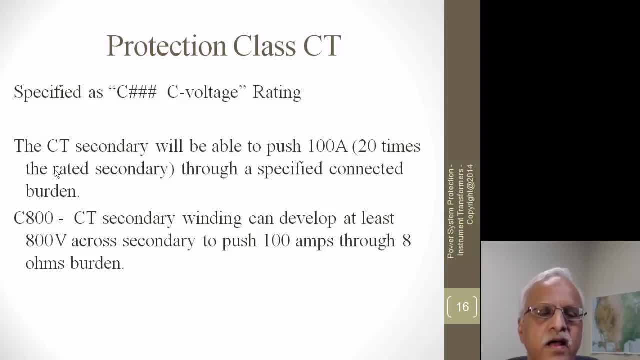 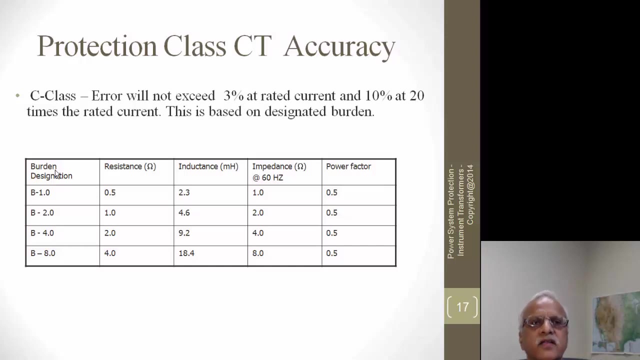 connected across is connected as a burden, and then 100 ohms is flowing through that 8 ohms. So this CT is capable of developing 100 or 800 volts to push 100 ohms through 8 ohms burden And whereas the burden in the case of protection class is defined little different than that. 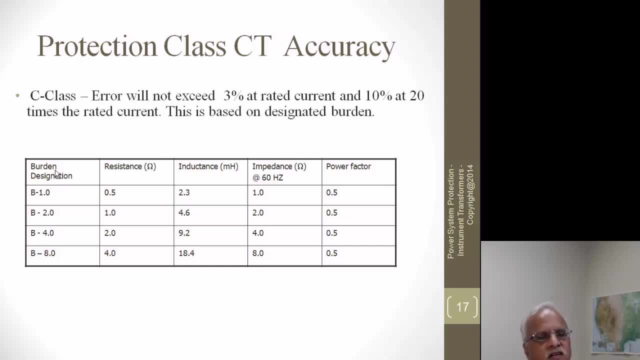 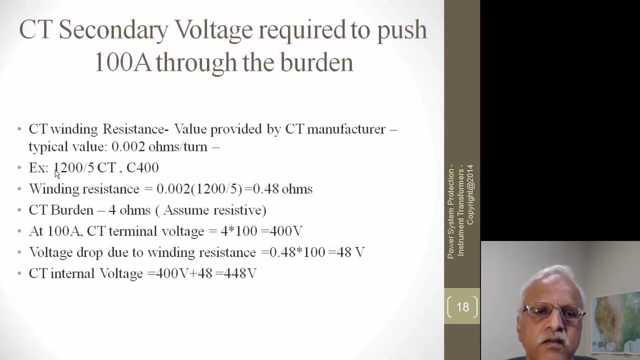 of the metering. Where mean metering? the power factor was 0.9, here it is 0.5. That means here we are connecting coils and all it might be more inductive in case of protection. Okay, and also, if you look at it, the secondary has a, has a winding which is normally used. 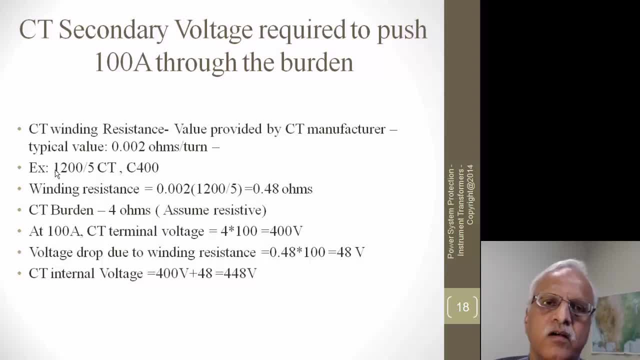 say a 10 gauge wire or a 14 gauge wire or a 12 gauge wire, depending on the rating of the CT. And here is an example where we have taken 1200 to 5. The primary number of turns is only 1. So the secondary number of turns has to be 240, which is the ratio of the currents. 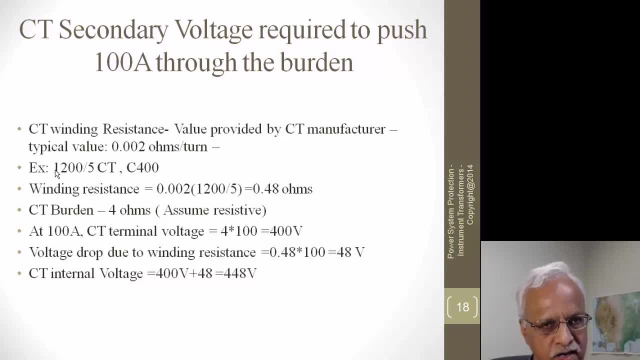 1200 to 5.. And now this winding, it could be a 10 gauge wire, or whatever gauge wire it is, It has some resistance, Okay, Okay, So the current that we are supplying is CT will provide this information And typical. 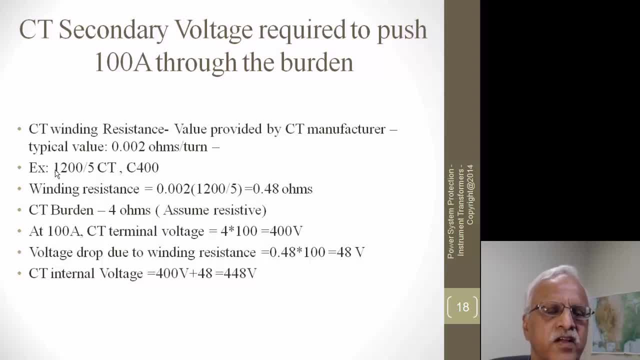 values are around 0.002. I have taken it could be very. it could be higher or lower than this number, but I've taken this as an example. So the resistance offered by the winding itself is about 0.48 ohms. 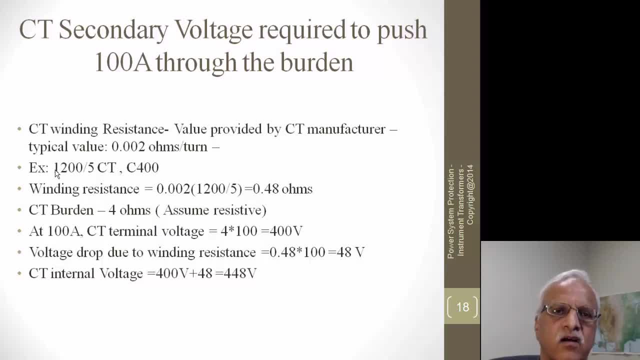 So if you have a resistive burden of 4 ohms connected on the secondary side and I know that this has to develop 400 volts to push 100 amps through 4 ohms burden, So the internal voltage that has to be developed inside the CT is 448.. 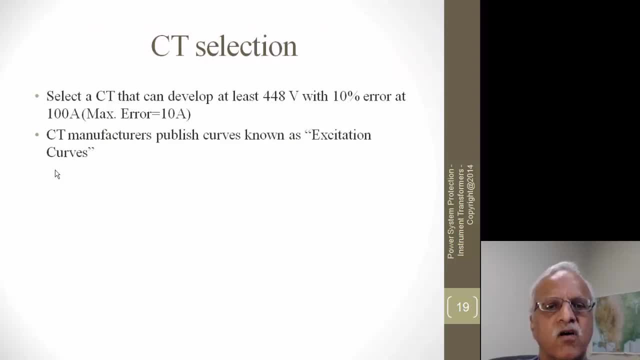 The CT manufacturers provide curves called excitation curve. And then the second thing here I want to tell is that if it is 100 amps flowing through, that the C rating also specifies that accuracy the error cannot exceed 10% of its rating. So if it is 100 amps it has. 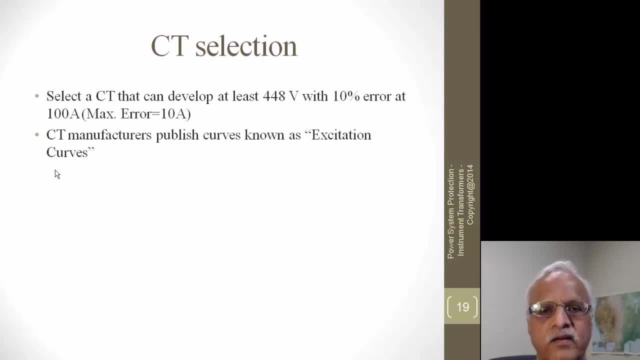 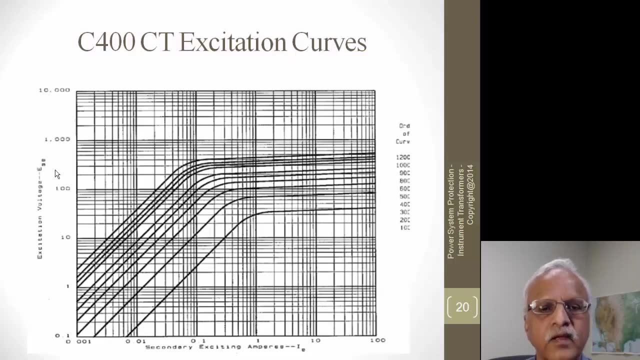 to be 100 minus 10, 10% of that is 10 amps. So it has to be 100 minus 10, 10% of that is 10 amps. Okay, So it has to be within 90 amps to 100 amps. 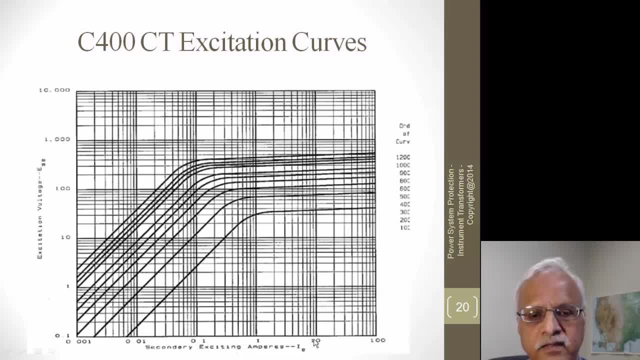 So now here, if you look at it, the excitation current is 10 amperes. So if it is 100 amps flowing and then 10 amps with excitation, then the voltage that is developed across the secondary side is given by this, which is about 600 volts. here You can go through. 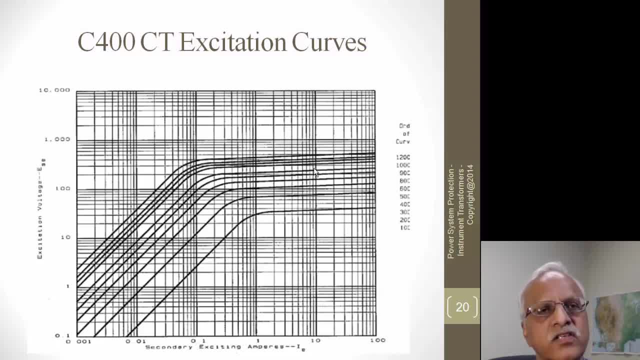 and look at it. So what it means is the internally, the whole CT can develop about 600 volts and then push 100 amps through the burden connected to that, which is 4 ohms in this case, And then the accuracy is error. 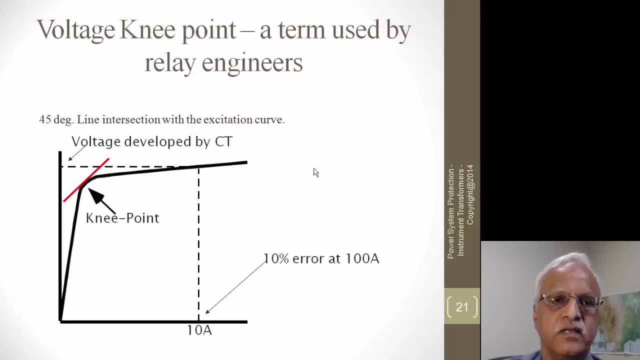 is less than is 10% or less. There is another term used by relay engineers: knee point. What it says is that the CT remains a linear up to that point, and then it starts saturating about that point. The American National Standards defines it as a curve, as a line, which is given by the C rating. 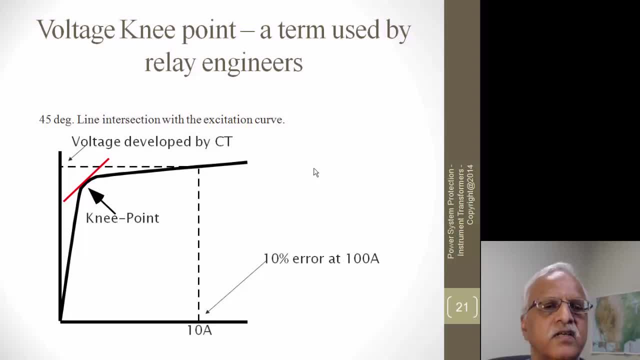 Which is given on the CT excitation curve, And then it is at 45 degrees And that point is called the knee point. And then you know, as you can see here, if you keep on apply a voltage to the secondary side and keep on increasing it, it linearly goes up to some. 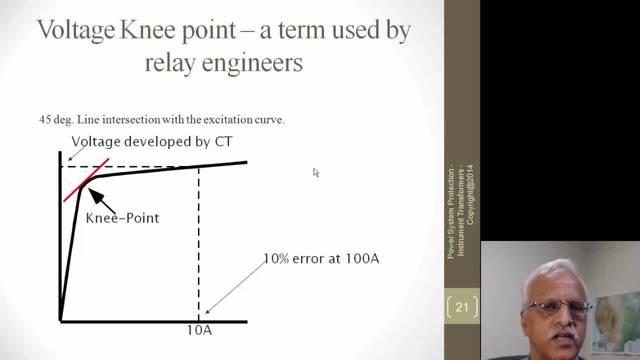 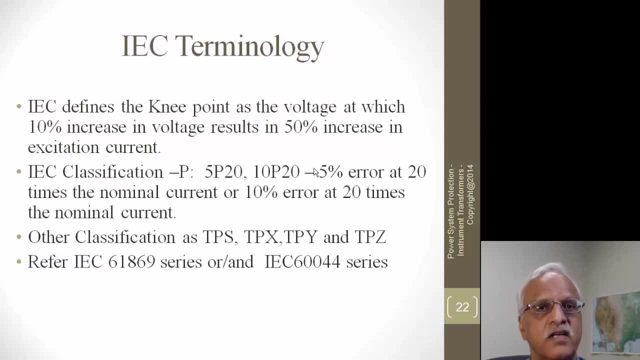 point afterwards. A little change in voltage will increase in a much higher rate of change of current. IEC defines using that equation. So it says that 10% increase in voltage results in 50% increase in excitation. current is specified as a knee point And below that it's almost linear. if you look at the previous excitation, 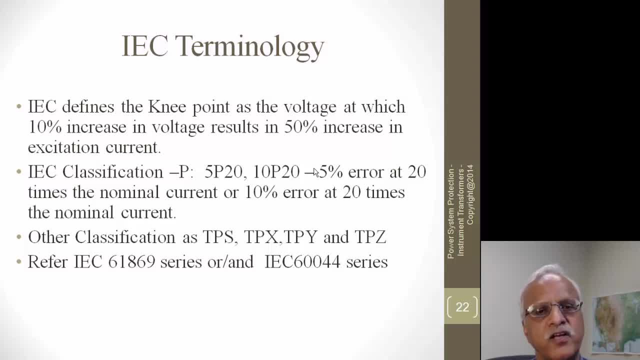 curve And IEC has other classifications: 5p20, 10p20.. What it means is it has 5% error when the current is 20 times the rated current on the secondary side, A nominal current. And then 10p20 is 10% error at 20 times the nominal current. 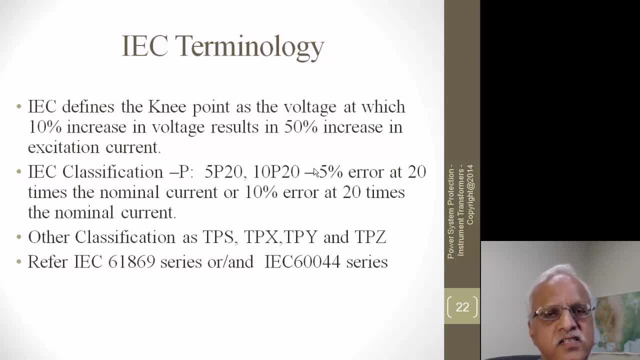 There are a lot more detailed classifications in IEC which I am not going in here. It is TPS, TPX, TPY and TPZ. Please refer to the IEC standards documents, which explain this in much more detail. 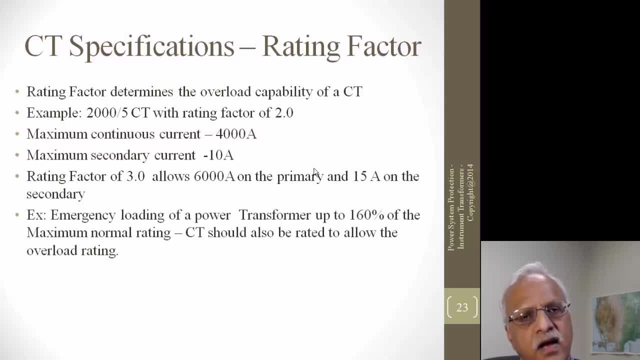 There is one more factor which we look at in the rating factor. As I mentioned earlier, a transformer can get overloaded. Ah, A transformer can get overloaded, you know, to 160% for a short time. So the CT also should be able to carry that much current. For example, if you have 1000 to 5 CT, and it can, the 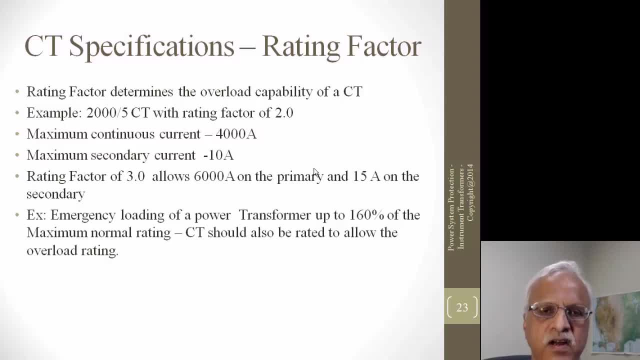 primary side current can go to 2000 amps for several hours. the secondary side current will be 10 amperes, So the 10 amps is going through the winding of the CT, which has some resistance. It produces some heat. So when you design a CT you specify the rating and then you limit this voltage rise due to 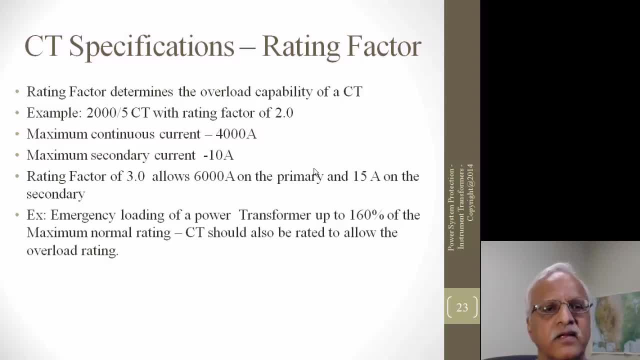 the current flowing on the secondary side, And then that is how the primary rating factor is defined, as the current that is going on the primary side. Maximum continuous current for a 2005 with a rating factor of 2 is 4000 amps. So the 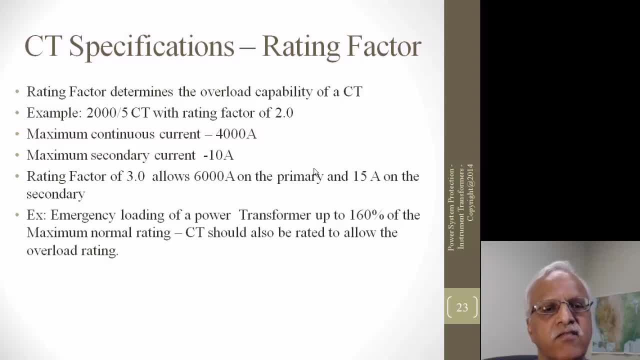 current on the secondary side will be 10 amperes. Ah factor of 3 allows 15 amps on the secondary side. so you know this is a good example. you try to use it in metering also. we know that in the meters 10% has higher error dot twice the error than at 100%. so what we do is yeah if it. 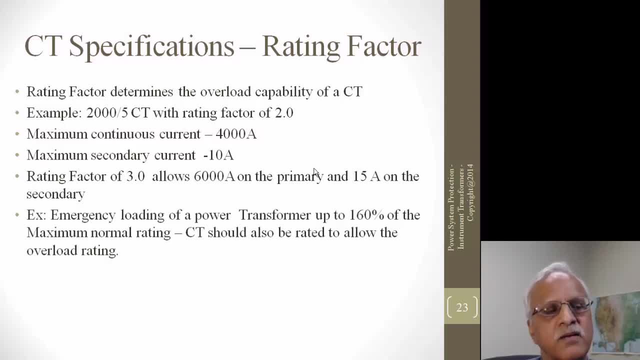 is a 2,000 amp circuit. we try to use a thousand amps, two thousand to five CT with a rating factor of two. so at 100 amperes it will have say, if it is a point three B one and thousand to five with a rating factor of two at thousand. 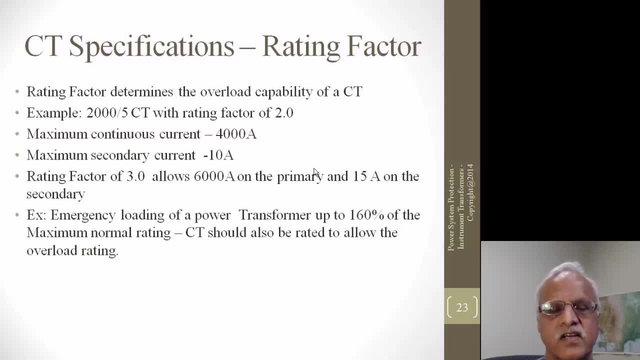 amperes it has point three percent inaccuracy, whereas that you know, at ten, a hundred amperes it will have an inaccuracy of point six percent. but at two thousand amps, when it is fully loaded, the CT is capable of handling that overload but its accuracy will still remain at point three percent. 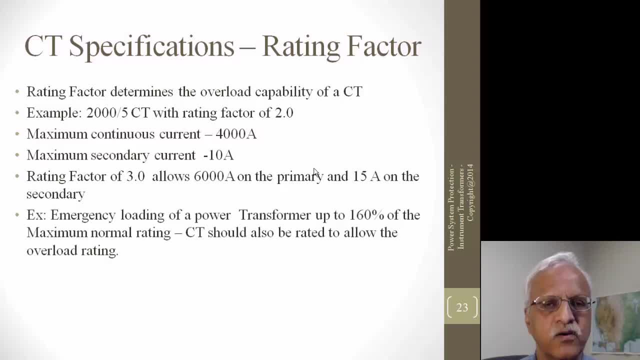 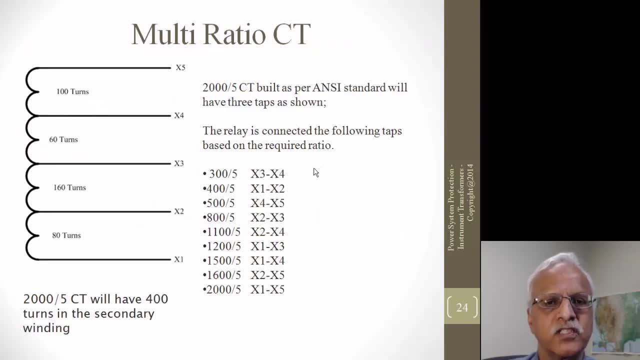 you can see that the accuracy of the accuracy, of the accuracy of the accuracy. this is very common in metering, where they use a lower ratio to to reduce the errors at very low currents and then most of the protection class are defined: where has got taps so you can adjust the CTs, and this is one of the examples I 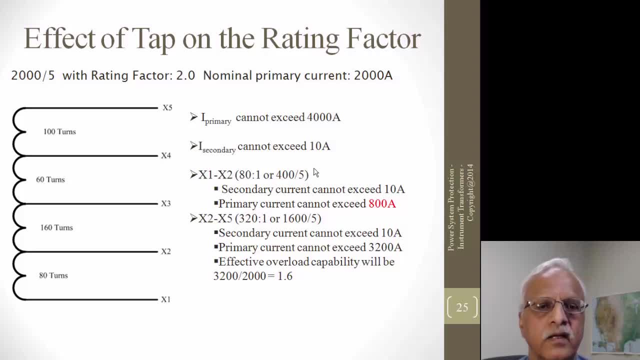 have given here now effect of this tapping on the CT, if you don't use a full rating, if it is a C 800, if from X 1 to X 5, then X 1 to X 3, I will be. they just the ratio of turns to the total number of turns that 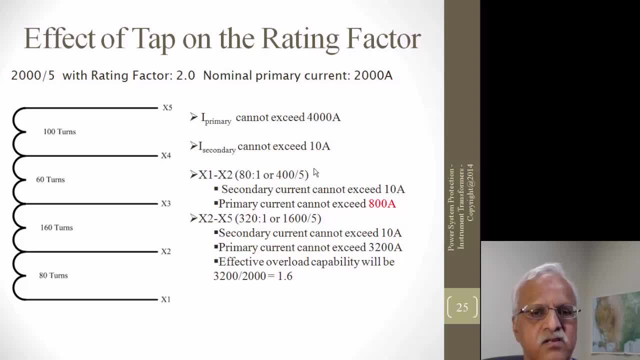 will be the voltage that will be developed across this, so your C rating also reduces and then also your rating factor reduces, as I mentioned, if it is two, and then the current on the secondary side will be 10 amperes, and then that still is limited by the type of wire that is used for the winding. so 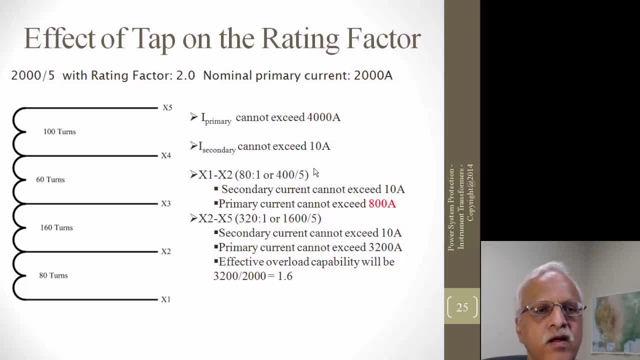 if it is that, you know, if in this case it is 400 tons, then if it is 2005 it can carry 4000 amps on the primary and 10 amps on the secondary. but if it is you know, it's only 80 to 1. if you are using that, the primary side, secondary side- 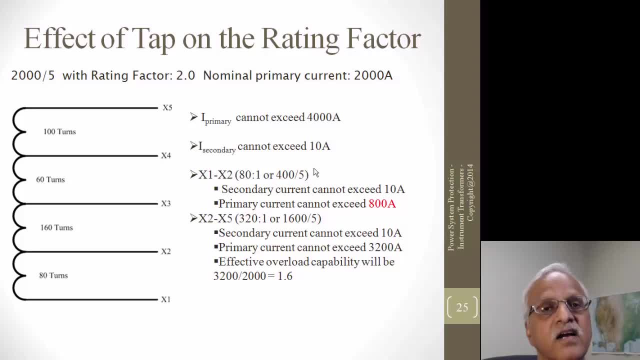 is still limited to 10 amperes, so the primary current cannot exceed 800 amperes. The other example I've given here is 320 to 1. the primary current cannot exceed 3200 amperes because the secondary one current will be limited. And the other point I want I made here was if the C rating 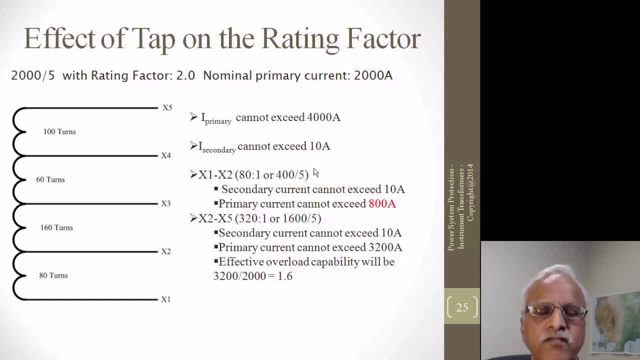 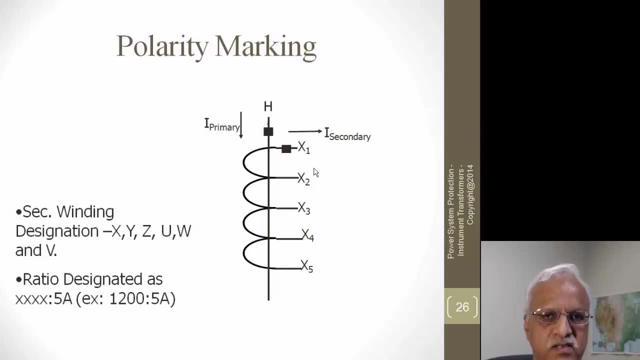 is 800 for the full winding. if you reduce it to 50 percent of the winding, C rating also reduces to 50 percent of that, because it is just the ratio of number of turns. The third one which we want to look at is the polarity marking. This is very important when 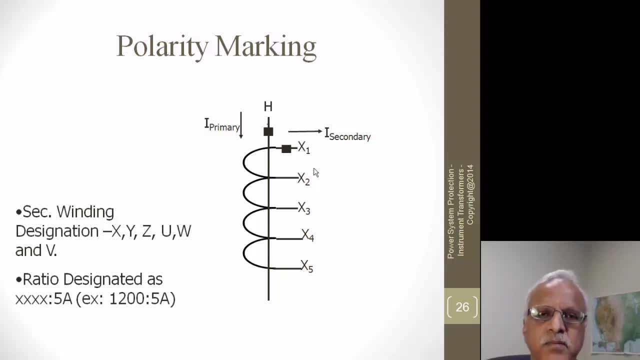 you have directional relays or when you are trying to protect a bus, where the sum of all the currents must be in the polarity. So if you have a bus that is in the polarity, then you have to be equal to zero, your directionality. how the current comes into the relay is also very important. 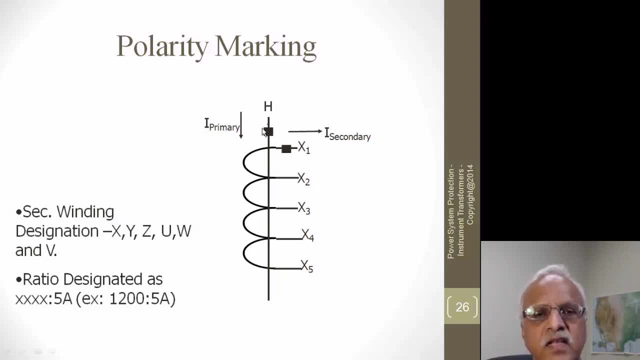 So you have a polarity marking convention. when the current enters this polarity marking on the primary side, the current leaves the polarity marking on the low side, and then you have different designation valve numbers, which is given by that. if you have multiple cities, then they are used X, Y, Z, W and especially in freestanding cities you have five cores or six. 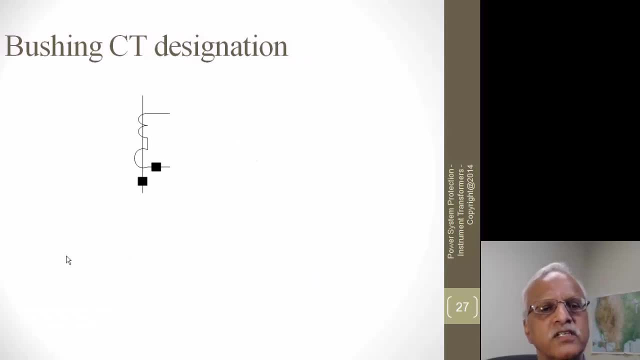 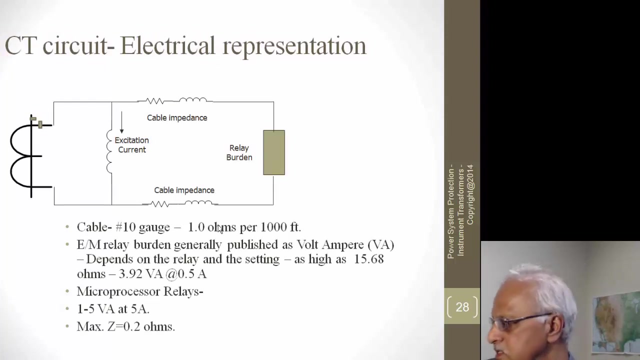 cores. you can use this. Bushing. cities are also designated with the hump, as shown here, as shown here, that is also specified, shown in the drawings. If you look at electrical parameters, if you look at electrical representation, I have a city here and then I know that there is some excitation current. 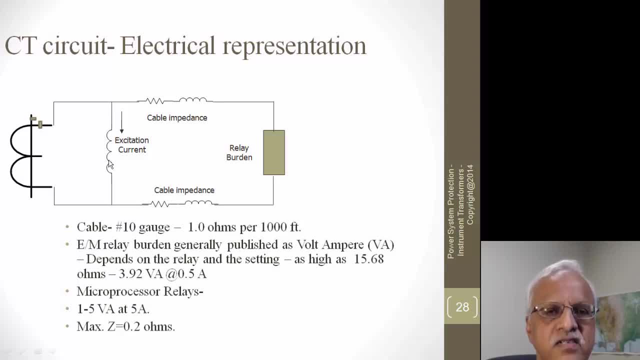 I can represent it as a shunt across the secondary side winding. and then you have got a cable impedance, which could be just a cable, it could be number ten AWG, and we just got a resistance of 1000 ohms per thousand feet. ohI am sorry, 11 ohm per thousand feet, not 1,000, and also it is on there. 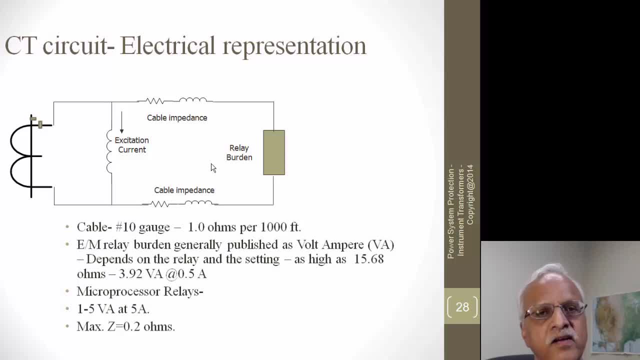 dependent on the temperature. if the temperature is a little higher in the warmer climates, they use about 1.2 ohms per thousand feet for that. It is not 100 ohms, but it is about x1 ohm per thousand feet for that. 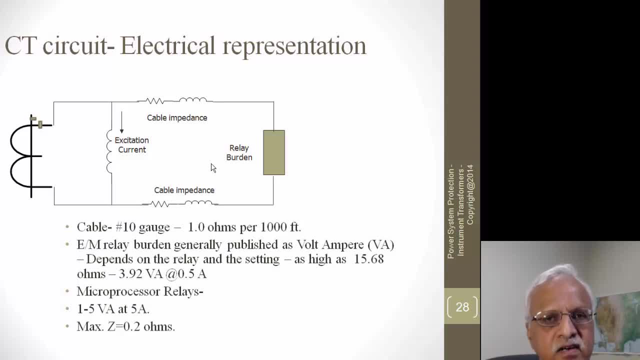 Electro-mechanical relays generally have a higher burden. it offers a higher impedance. so it depends on the relay and the setting. it could be as high as 15.68 ohms, you know, and if you have 15 ohms and if you have 100 amps going through that, then you have 1500 volts developed across. then the CT is only 880 points saturated. 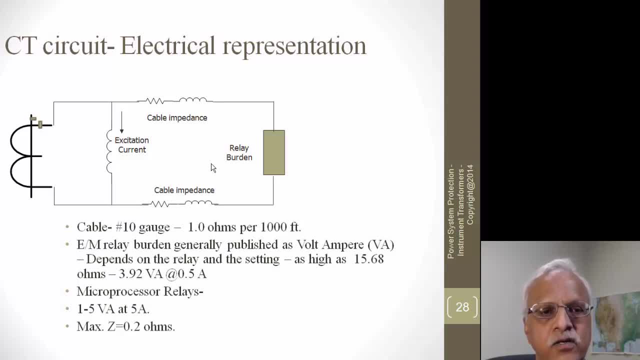 So higher the burden, there is a likelihood of the CT saturation also, or CT not reproducing the waveform as we need for this. In the microprocessor-based relays the burden is very low. it offers very low impedance to that and most of the times when you use microprocessor-based relays it is the cable impedance that comes into picture and that is the one which determines the voltage across the secondary side of the relay. 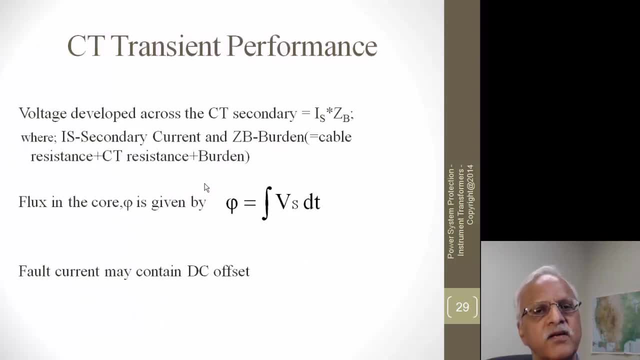 And then that voltage developed across the secondary side of the CT is the one which develops a flux in the magnetic core and flux is just an integral of that. and if the fault current has got primary fault current has got a DC offset and if you have a resistive burden as an example, in that example the voltage also will have a DC offset because it is current times, the resistance, and then and it gets integrated across the secondary side of the CT. 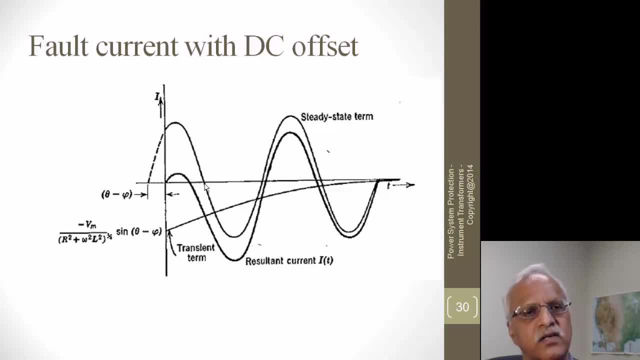 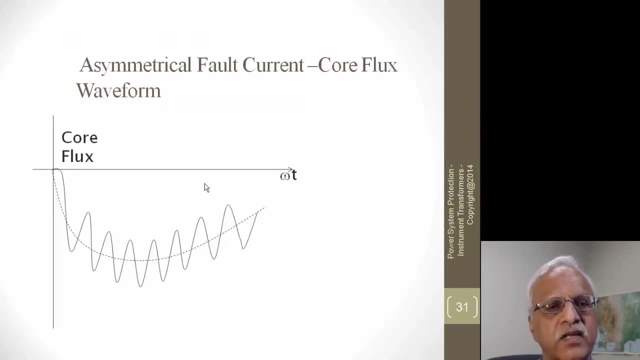 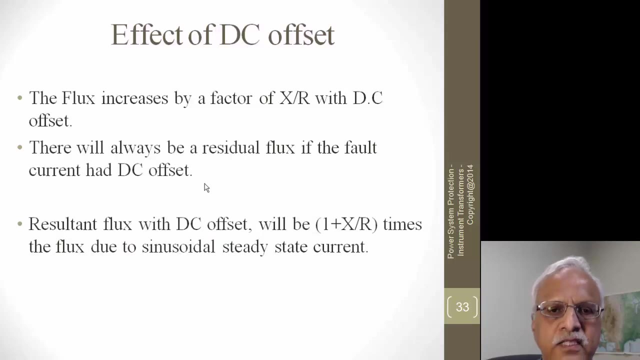 And then it gets integrated with that and then it produces much higher currents. this is just showing the primary current and then this is the flux, how it develops inside the flux, and that flux can reach very high values. and then let's go to the next one. the flux increases by a factor of X over R of the DC offset. so if the voltage is just with a DC offset, which could be maximum 2 per unit of the DC offset, 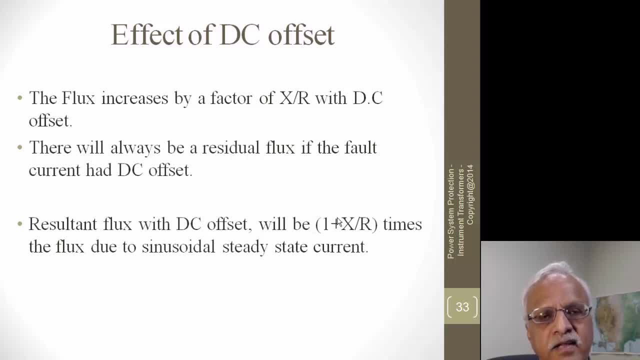 the current can go, it can be fully offset and then the voltage also can be fully offset because the current is going through a resistive burden, as an example. but if you integrate that then I get 1 plus X over R times the flux.